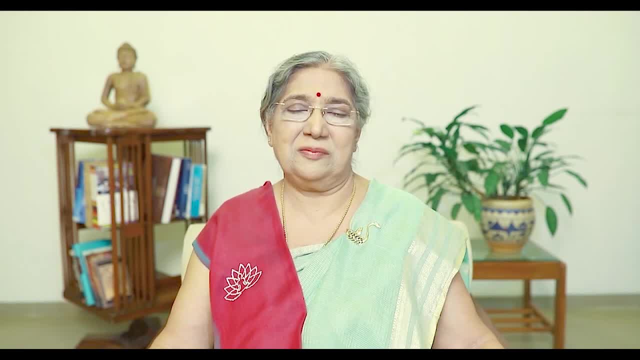 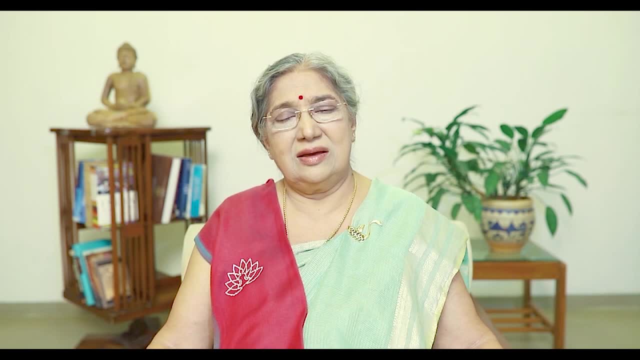 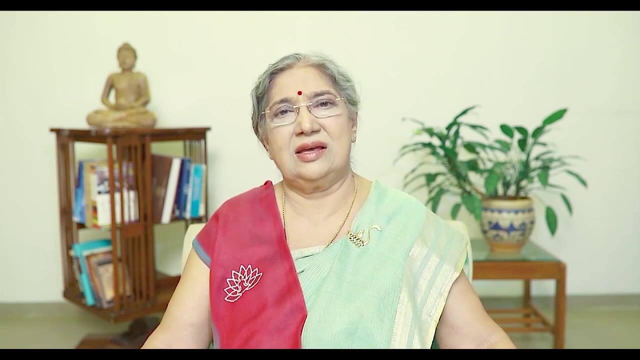 walk where the floor is not even Careful, because very often I have seen ladies falling down. Second, she should be learning to sit on the floor or cross legs and sitting. That also should be in a day, whenever possible. Little movement, sitting on the floor. how you clean the floor with a broom. 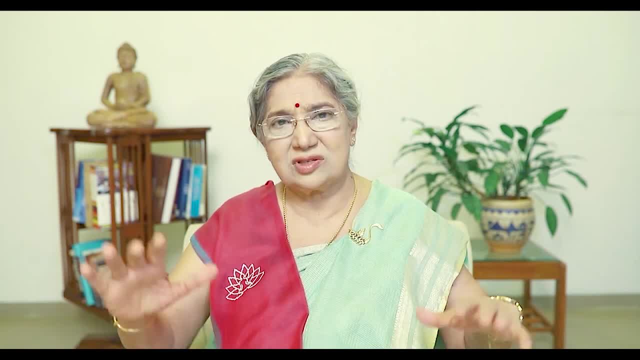 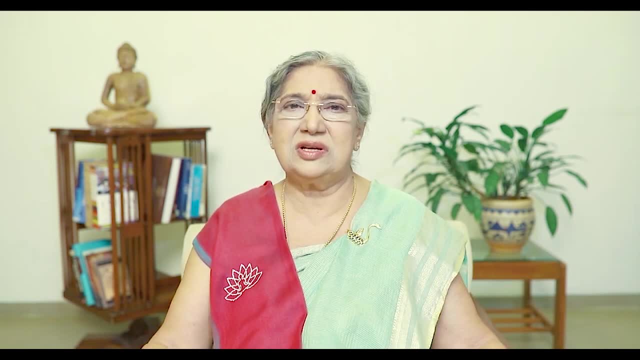 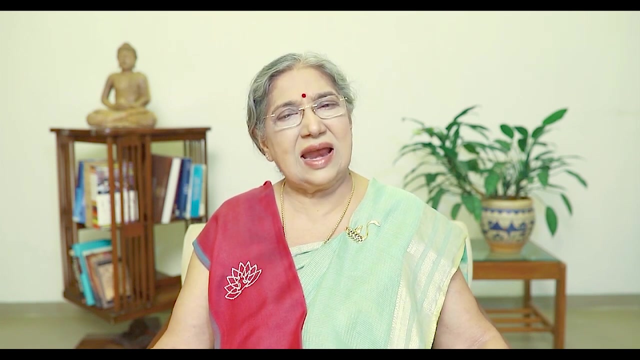 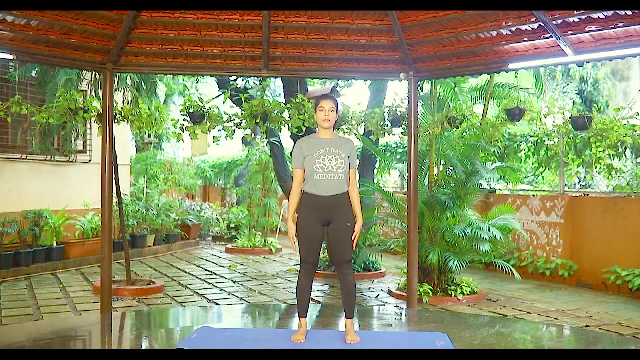 or wiping the floor. squatting down is most essential Till seventh month. person should be doing this. What I am trying to say is physically, person should be active. Now, certain asanas which person should be doing are: standing talasana: Both legs keep away from each other. Raise your hands up. 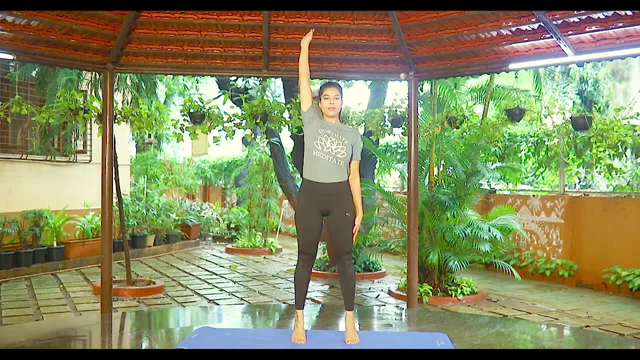 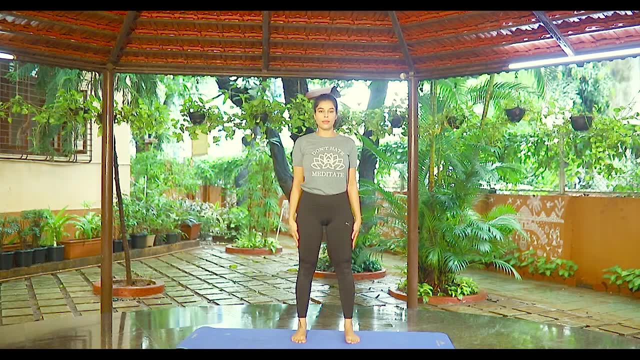 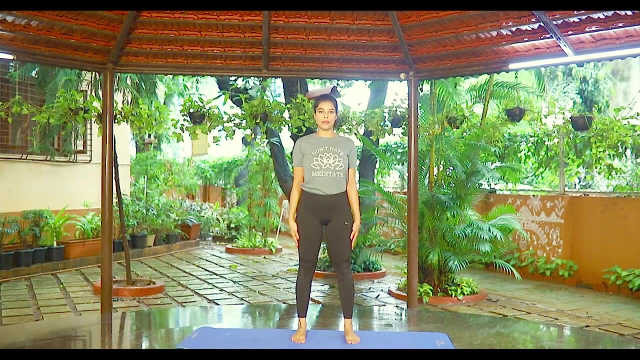 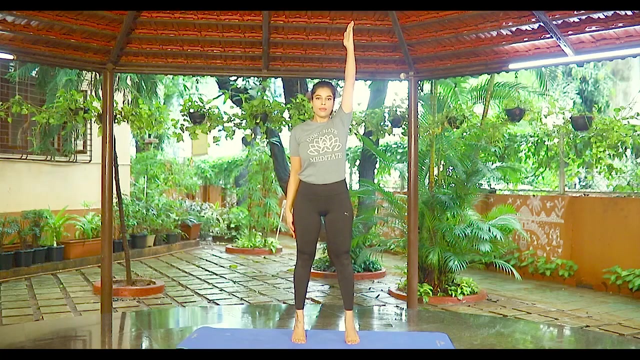 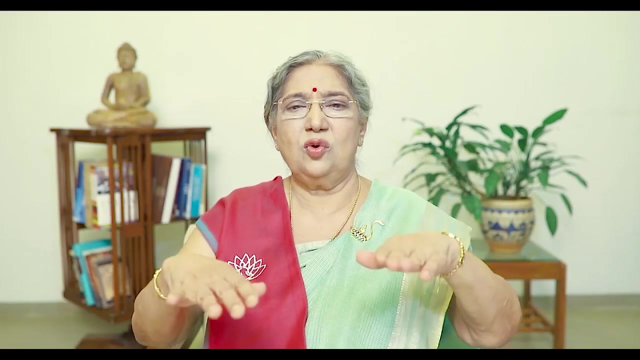 while breathing in and rotate your arm from behind exhaling. This rotation is important For seeing that the breasts are relaxed and firm. Other hand also going up: stretch, hold for six seconds exhaling. bring it down. You could raise on your toe up and down, Sometimes holding something. 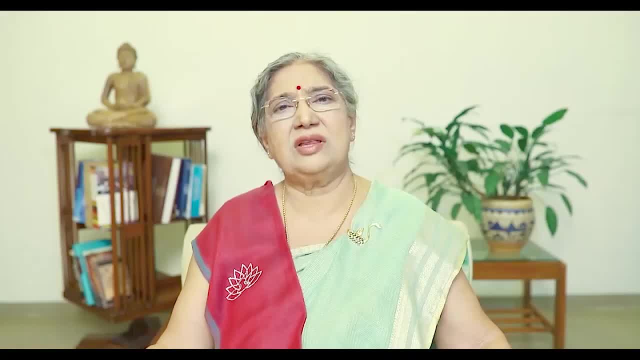 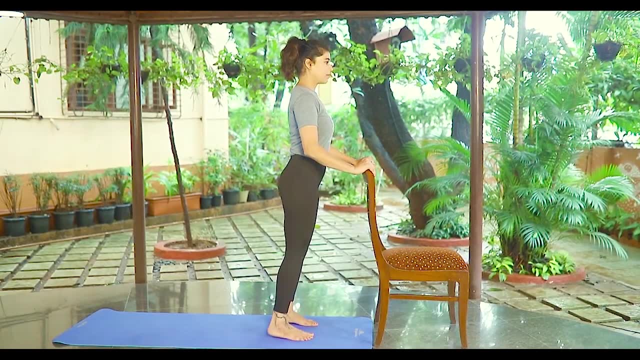 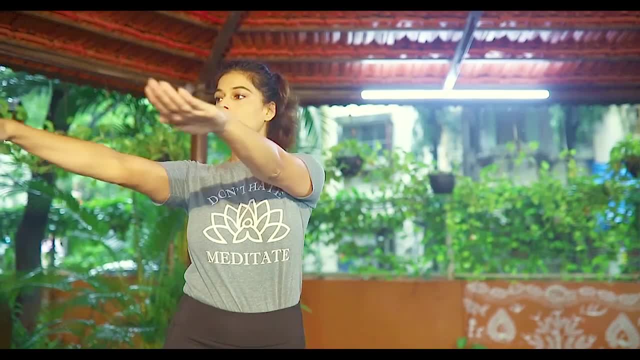 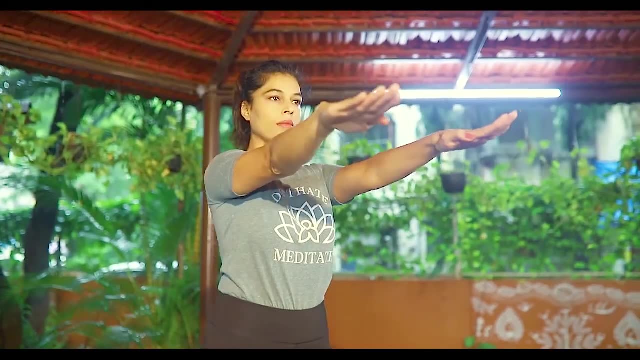 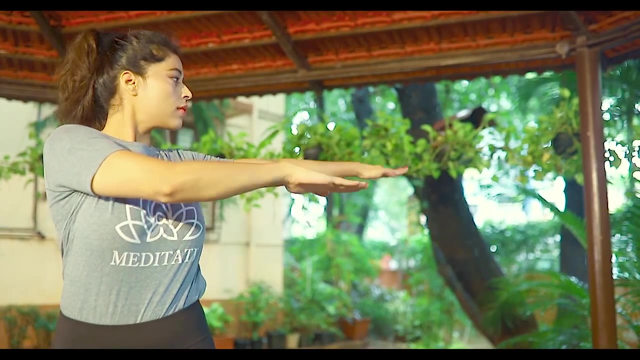 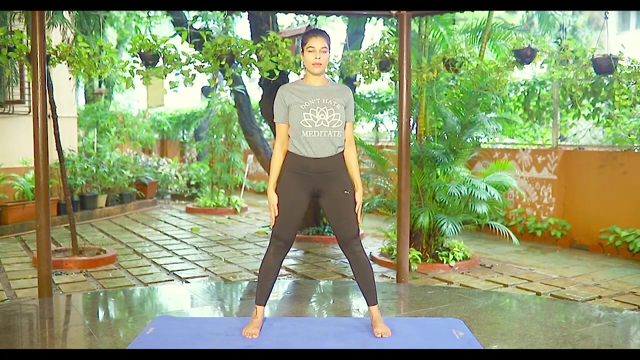 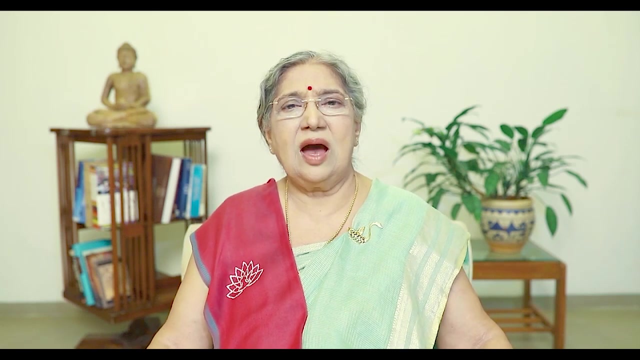 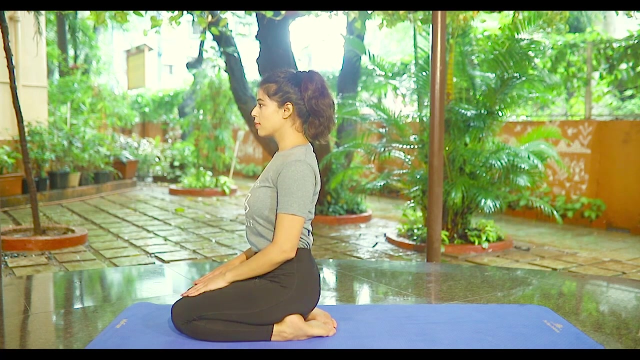 rotate your arm, that is, twist your hand behind. Look back, come back normal. Go on the other side. look back, come back normal. Every asana should be done once, or maximum twice, but not more than that, Preferably once. You are just bringing movements. Now sit, Let's do Ustrasana, camel pose Here. sit in Vajrasana. Take the support of 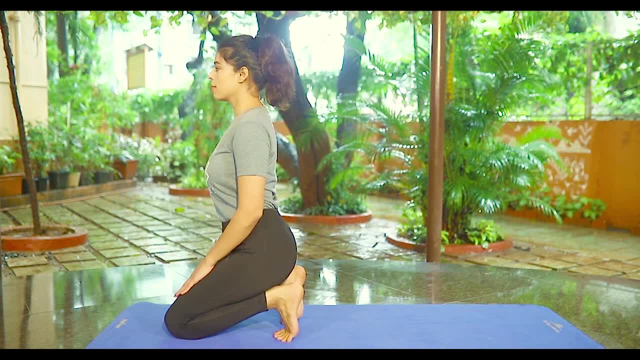 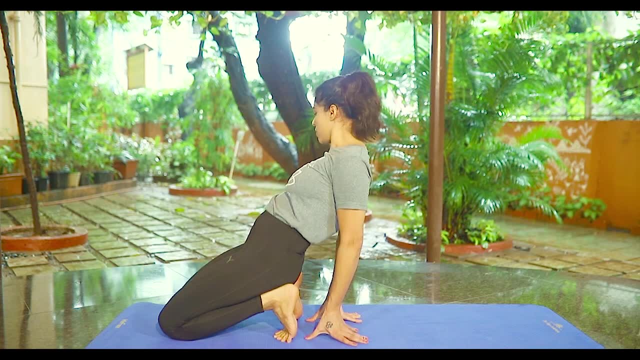 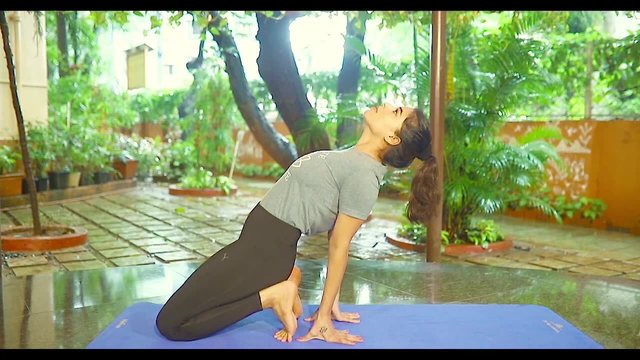 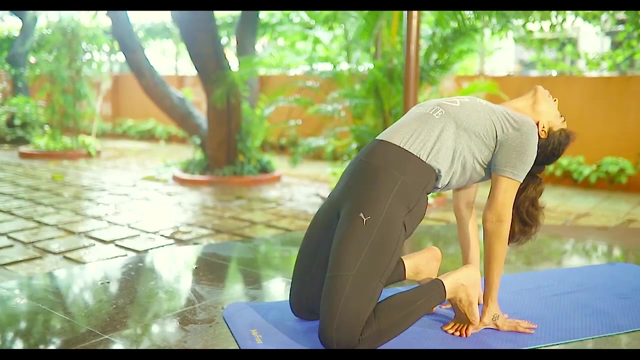 your heel behind And then lift your seat up, Push your head backwards, Inhale fully. Very good posture to see that there is a nice stretch on the abdominal region where the uterus sagging down will not take place. You'll bring it up. 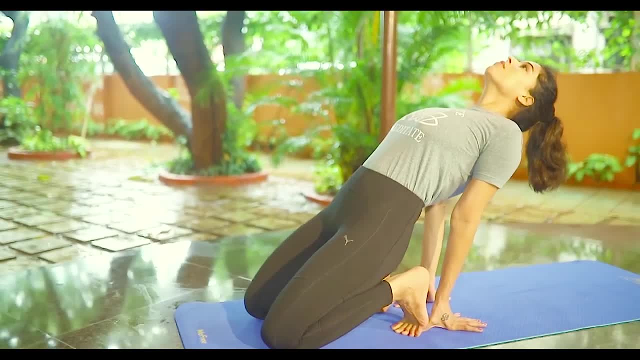 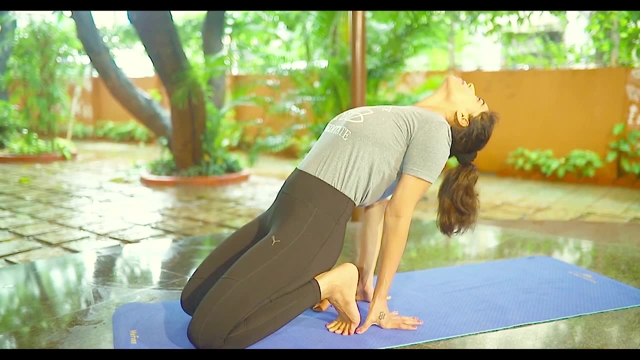 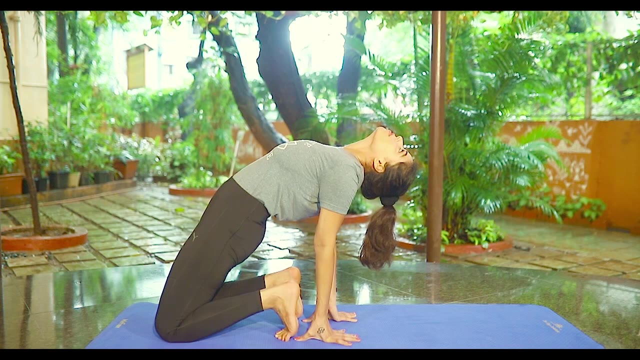 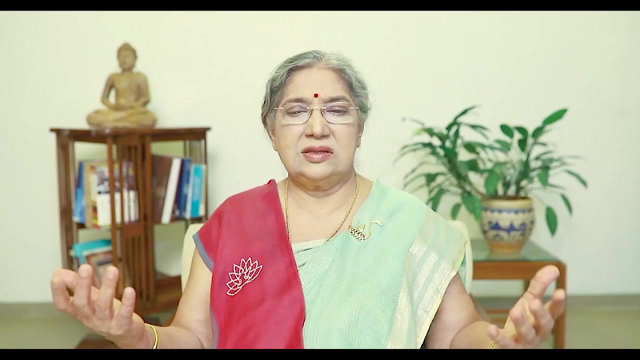 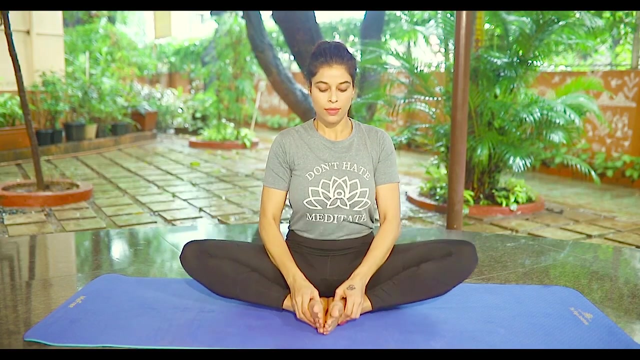 Come back to normal position Again. do the same. Take the support of your both arms behind to lift your body up. Do that, Stay little while and come back to normal position. Now sit with your legs together, maybe in Vajrasana position. Try and see that your legs are little bit. 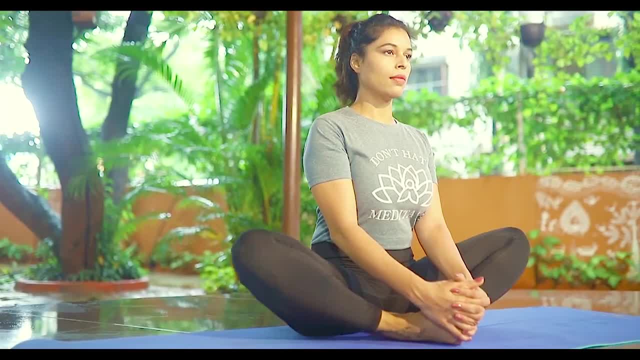 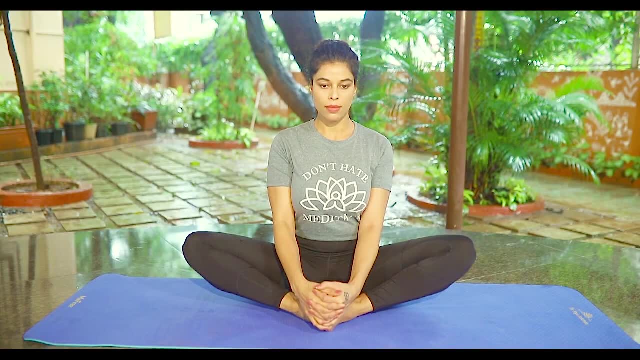 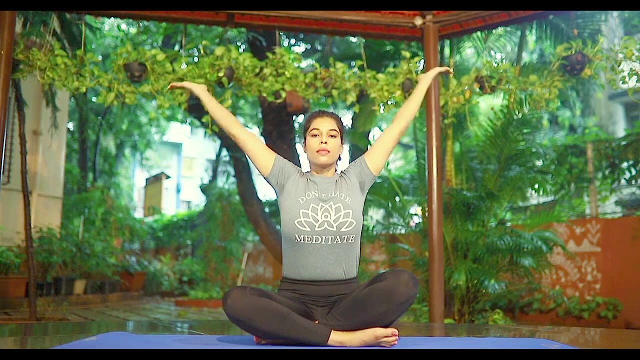 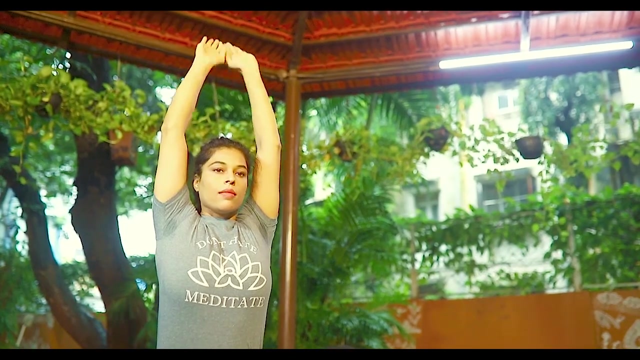 flexed Like a butterfly movement. Press it, Relax Vajrasana position. Sit in Sukhasana, Move your both arms up Inhaling Parvatasana Mounted pose And bring it back Again. try once Inhaling. Again. try once Inhaling Parvatasana Mounted pose And bring it back Again. try once Inhaling Again. try once Inhaling Parvatasana Mounted pose And bring it back Again. try once Inhaling. 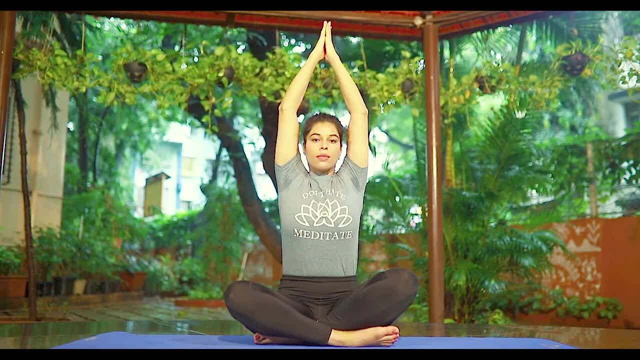 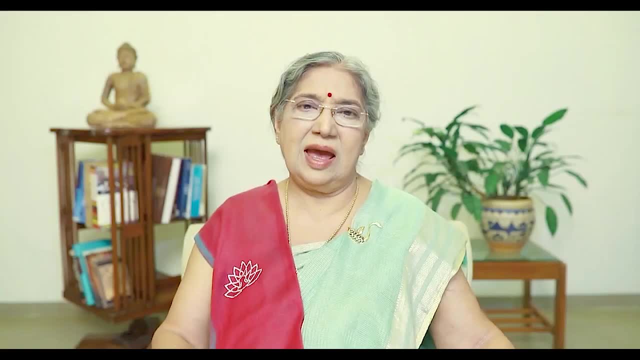 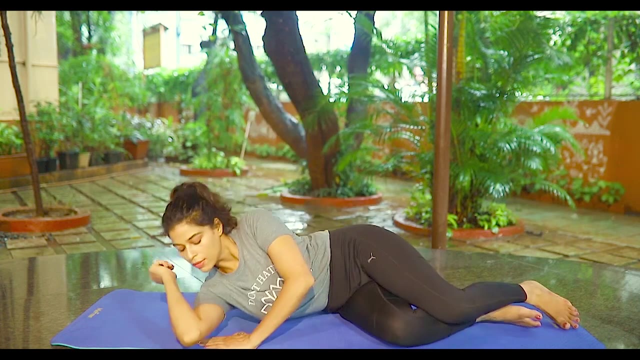 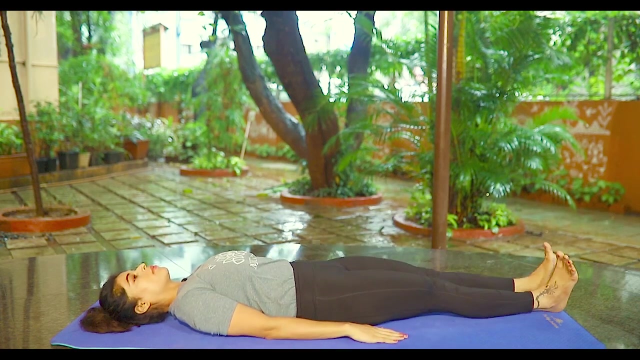 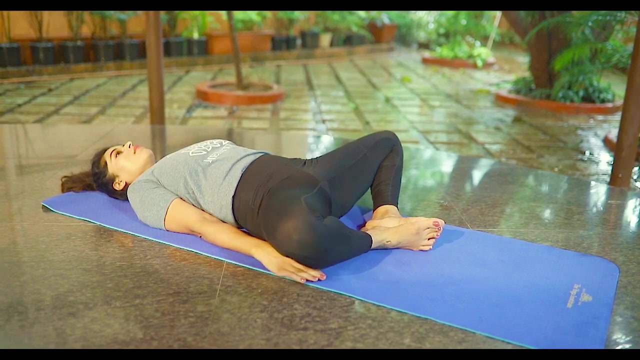 Raise your both arms up, Exhaling, Bring them down. Now lie down. While lying down, always turn to the side slowly and lie down, And in this position, do Bhadrasana again. Bring your both legs together, Fitting your sole, Doing Namaste with your legs. 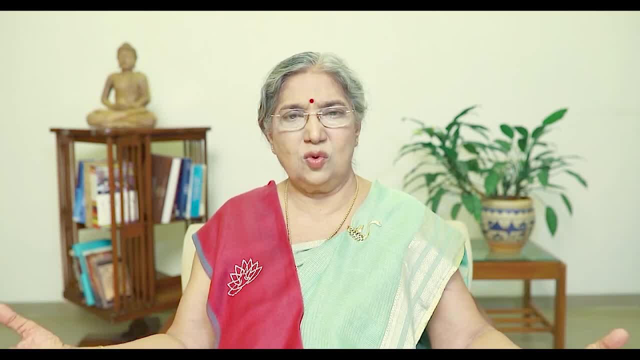 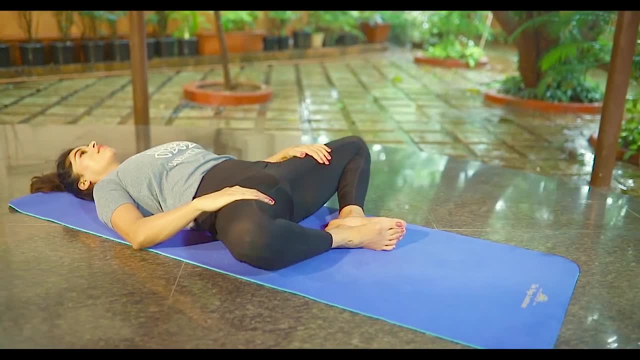 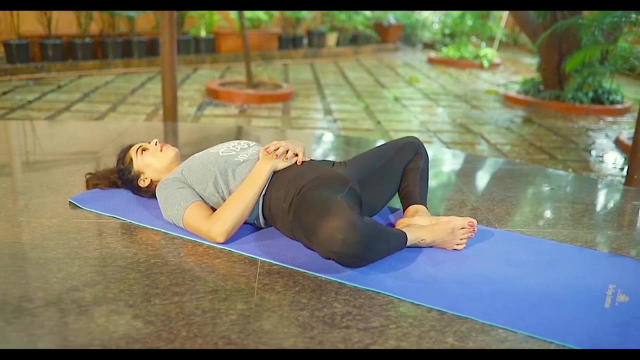 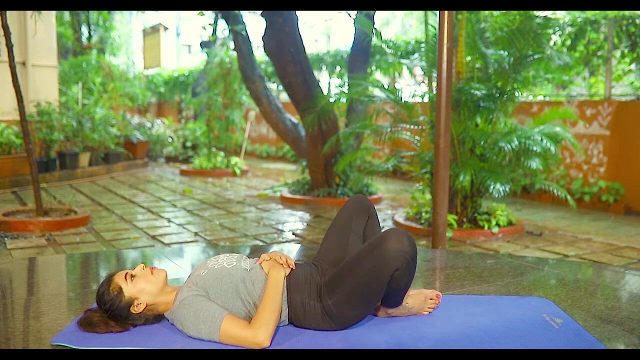 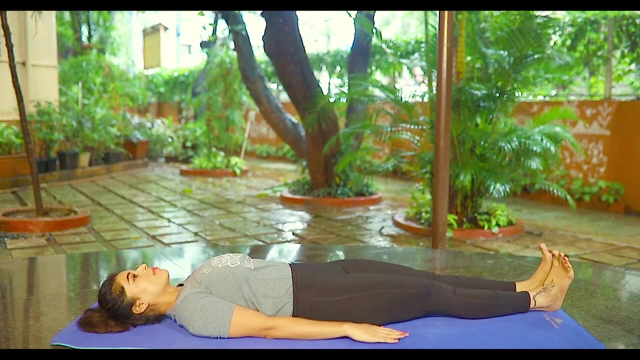 And trying to see that your knee is closer to the ground. Do little bit movements in the beginning, But not vigorously, Very slowly, And allow this posture for some time. Come back to normal position. Very often there is a swelling in legs during pregnancy. 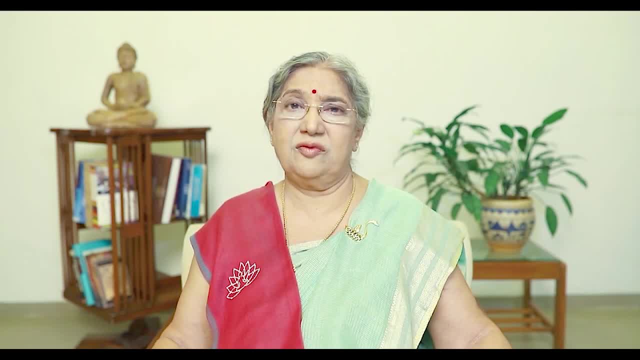 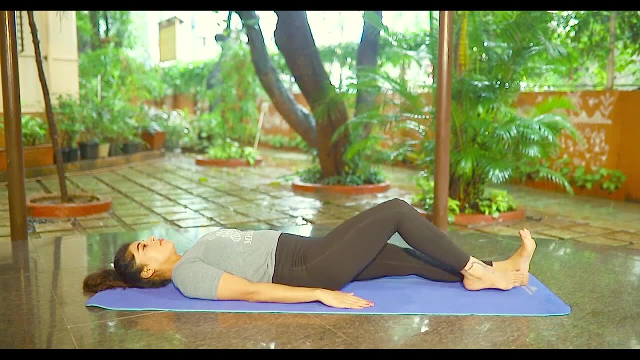 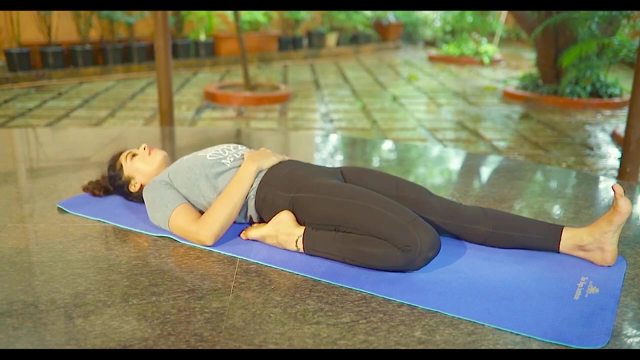 So this is a very good posture to overcome swelling. Lie down on your back. Fold one leg as if you are folding in sitting in Vajrasana position, From knee to the side, But not sitting on the leg. Leg around your waist, Around your hips. 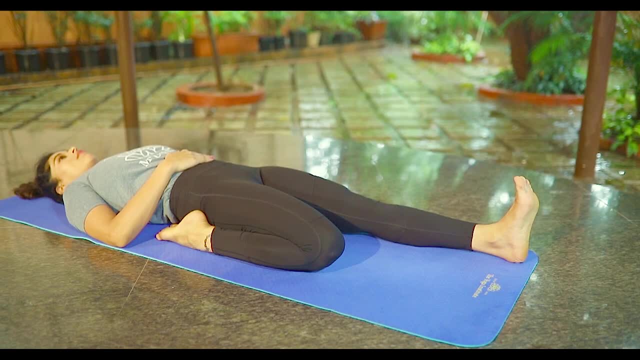 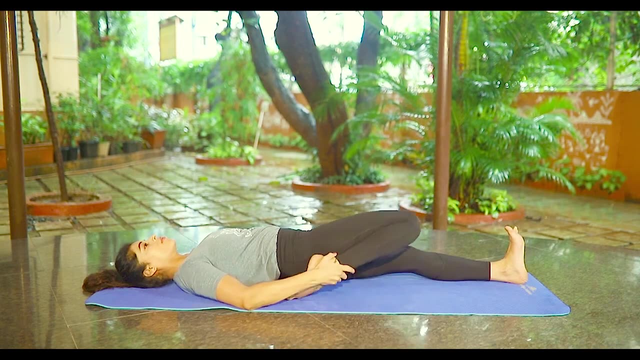 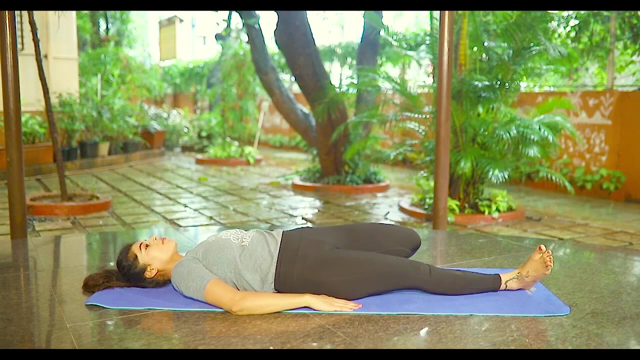 It is called as Pariyankasana. One leg at a time. Make it straight. Stretched again Straight. Take another leg, Fold it. Stay in that position for some time. You will have a good pull on your thigh. 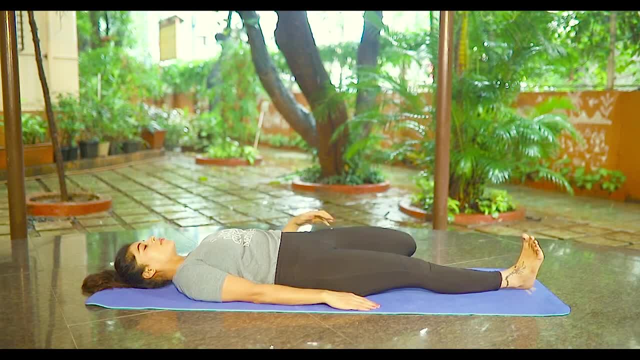 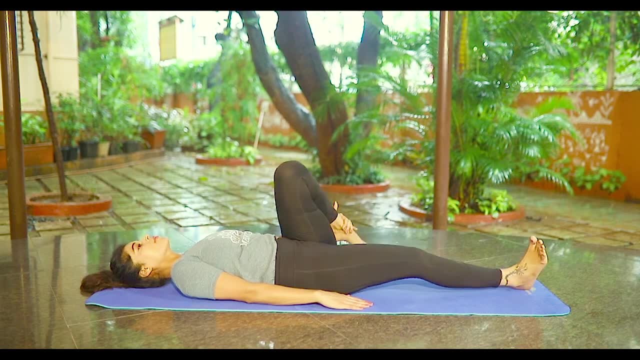 Come back to normal position. If it is very comfortable, then try with both the legs. If it is very comfortable, then try with both the legs. If it is very comfortable, then try with both the legs. Stay for some time And come back to normal position. 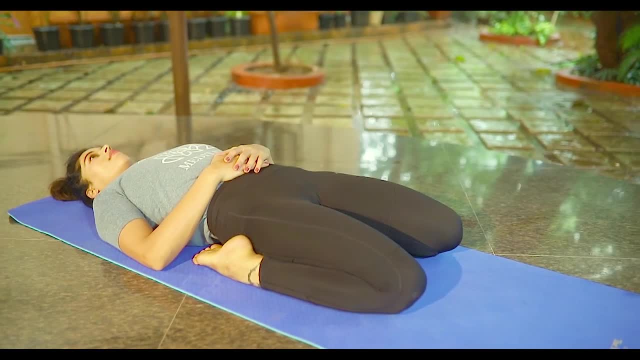 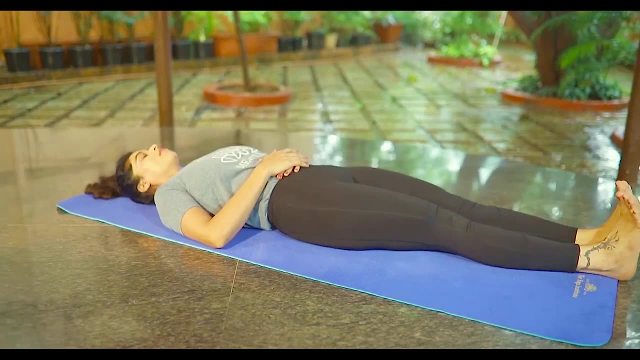 These are the movements which we are supposed to do. These are the movements which we are supposed to do. Do this with normal breathing. Your whole focus should be to see that you don't pull too much of your leg muscles. You are not used to it. 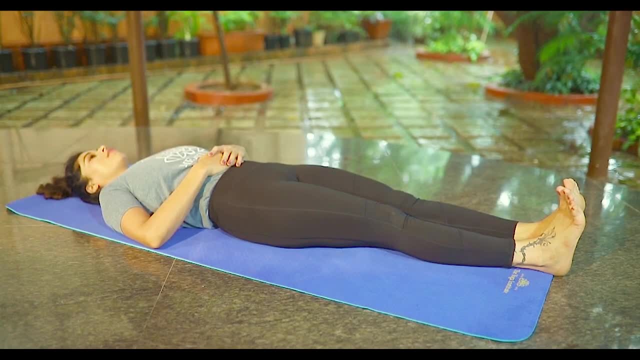 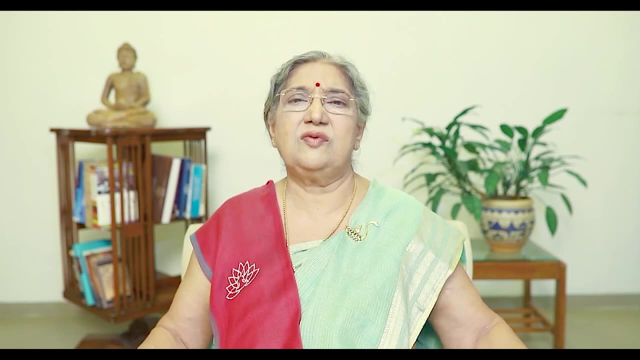 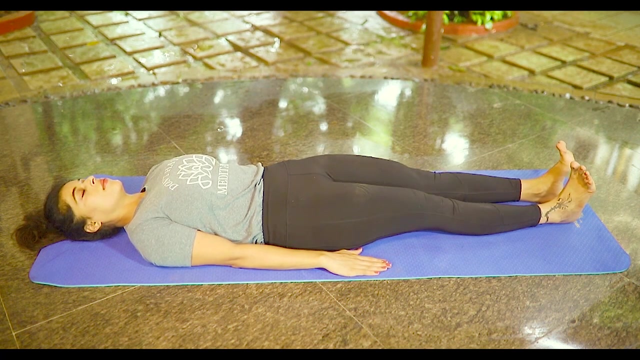 But practice this. This would really help. But practice this, This would really help. But practice this, This would really help. Hey, Stand up. You can remain sitting and move because you have muscle around your vulnerable muscle. You areками lying down in Padmasan position, which we call as Matsyasana. 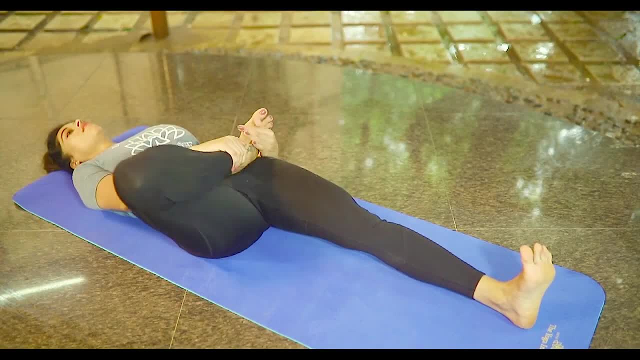 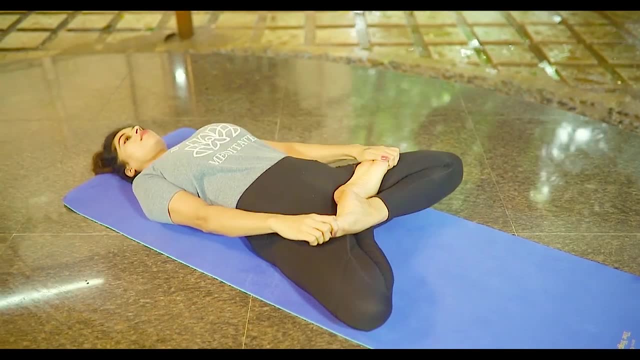 A very good posture for pregnant women. Cross your legs in Padmasan in a lying down position. Cross your legs in Padmasan in a lying down position. Good, pull, good strength in your lower abdomen. Good pull, good strength in your lower abdomen. 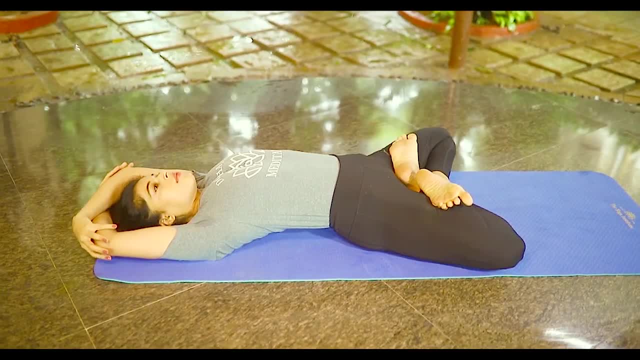 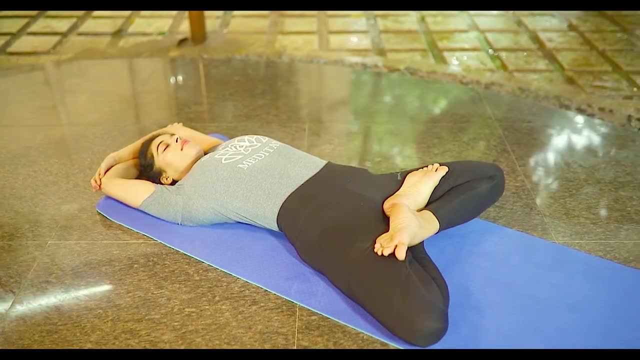 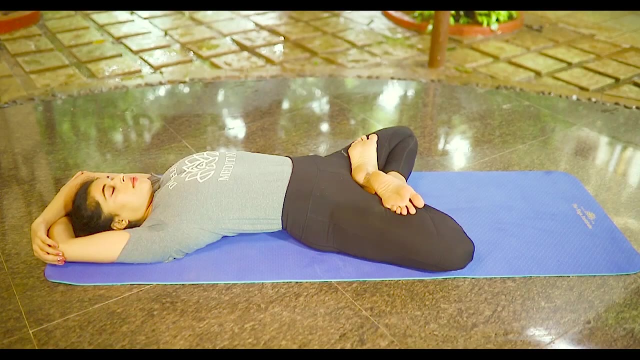 Stay for half a minute and leave it. Stay for half a minute and leave it. Stay for half a minute and leave it. so we are doing asanas, but not exactly with proper breathing rhythm and all we are doing it with a normal breathing and just moving our limbs here and there to maintain little.